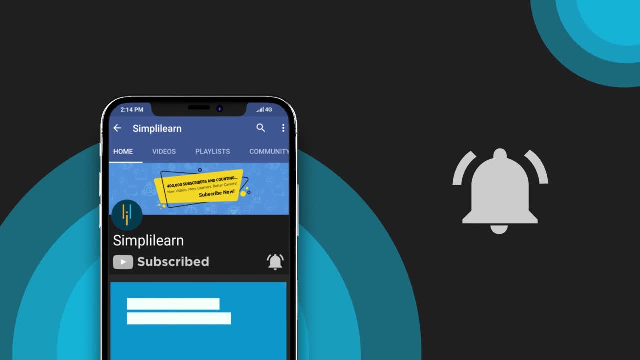 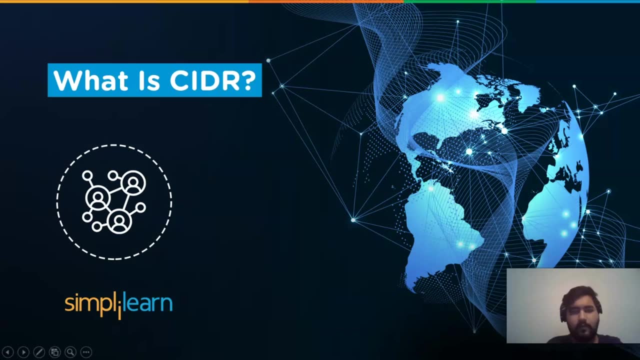 With the increase in the networking devices, either for professional or personal use, the need to access the internet to perform various activities has increased And, in this process, having an IP address assigned and then being routed to the network model and is applied using the classless inter-domain routing CIDR. 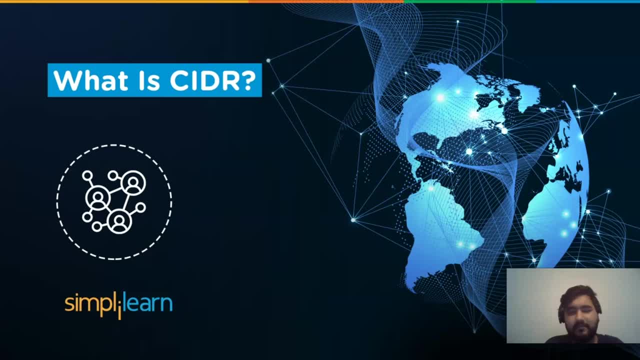 Hi guys, and welcome to yet another interesting video by Simply Learn. But before we begin, if you love watching tech videos, subscribe to our channel and hit the bell icon to never miss an update from us. Now, without further ado, let's take a look at the agenda for today's. 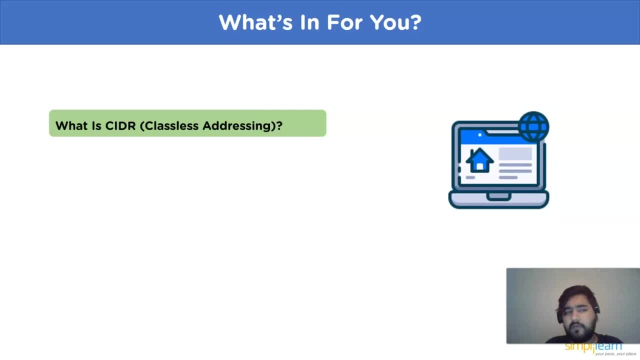 session. To begin with, we will look into what is CIDR, that is, classless inter-domain routing. Moving on, we will look at some of the rules to perform the CIDR, addressing, Continuing with the working of the CIDR And, at the end, 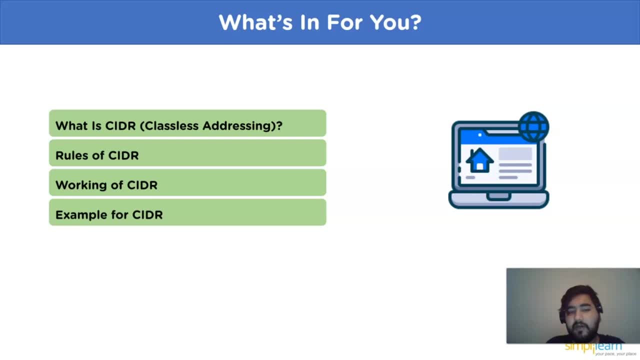 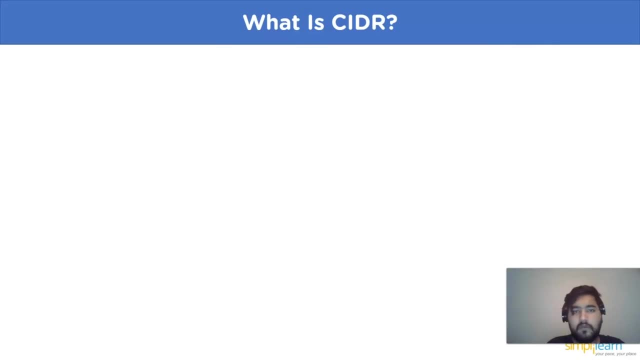 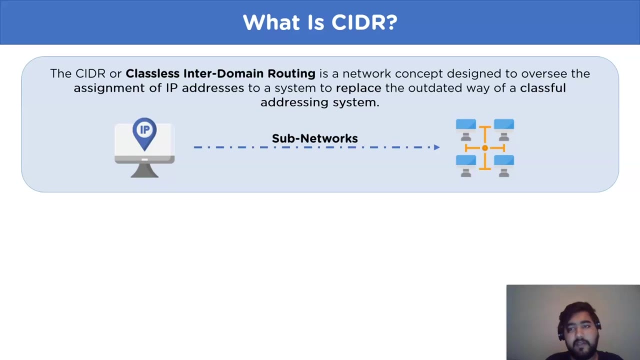 we will look into some examples to better clarify all the doubts we have learned so far. Now let's take a look at the first heading. that is, what is CIDR? The CIDR, or classless inter-domain routing, is a network concept designed to oversee the assignment of IP addresses. 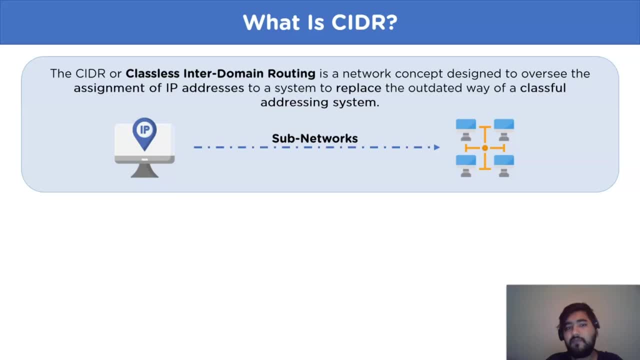 to a system. CIDR is a routed way of a classful addressing system. Furthermore, using the CIDR method, there is low wastage of IP addresses and it also is helpful in maintaining the routing table, and it performs the task of subnetting, which saves a lot of IP addresses. Now let's 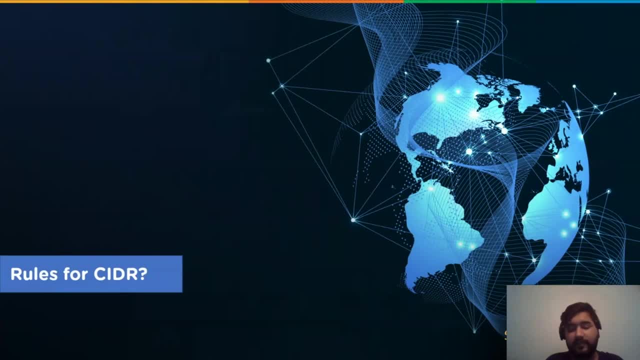 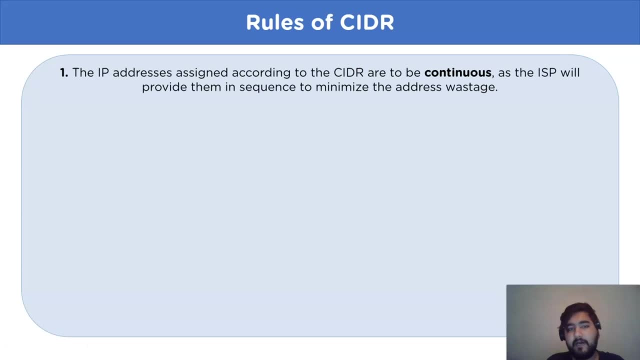 move on to the next heading, that is, the rules of using CIDR. To better understand the working of CIDR addressing In the later part, please take a look at the rules very seriously. Let's take a look at the first rule, that is, the IP addresses assigned are, according to the CIDR, are to be continuous. 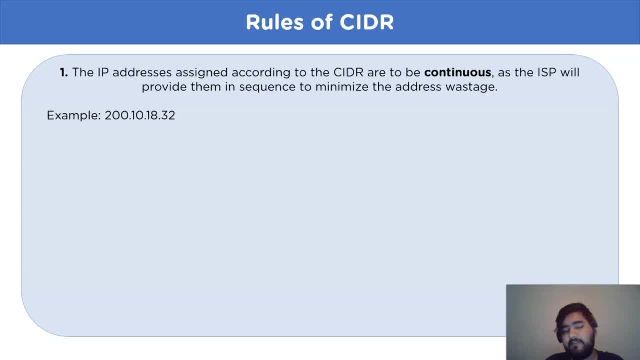 as the ISP will provide them in a sequence to minimize the address wastage. For example, if we have an IP address 200.10.18.32,, then the addressing will take place as 200.10.18.33 and moving on to the nth position, as mentioned in the example. This proves that 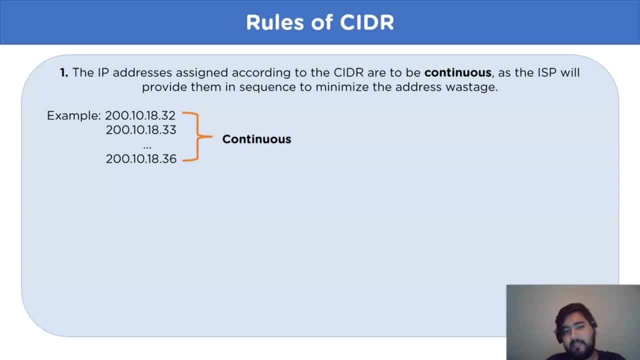 they are continuous in assigning of IP addresses. Let's move on to the next rule, that is, the number of addresses in a CIDR block is to be power of 2, that is, in case the number of addresses is odd, then it's invalid value. For example, 2 to the power 4 is equal to 16, where 4 represents the. 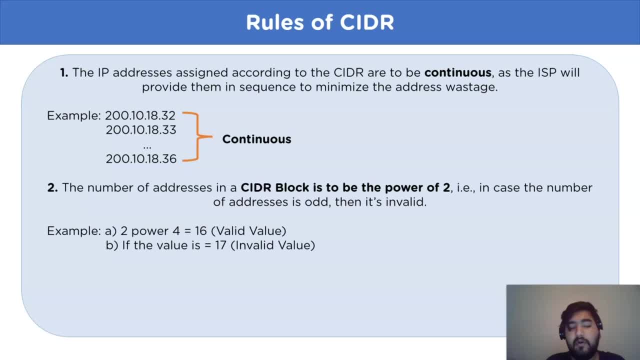 number of hosts, whereas if the value is 17, then it's an invalid value. As for the last rule, we have use of CIDR block for notation purpose. that is, for example, if we have 211.19.34 slash 28 as an IP address, then the block ID of 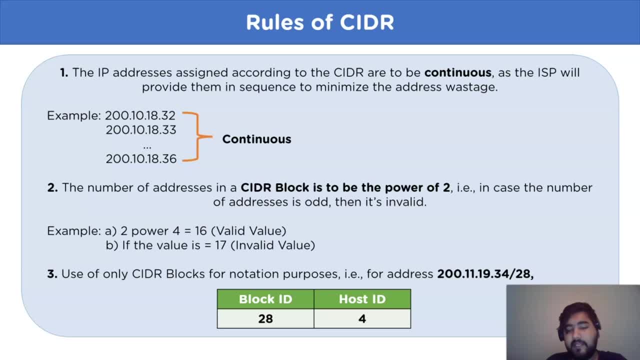 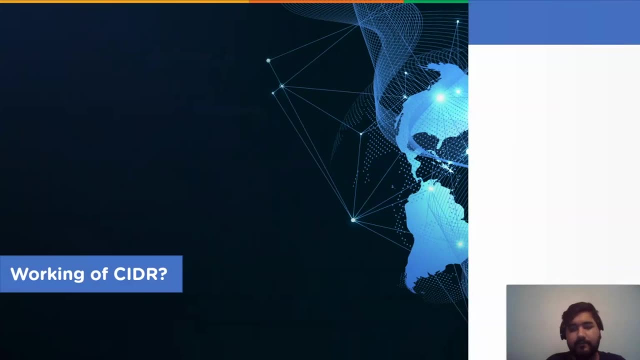 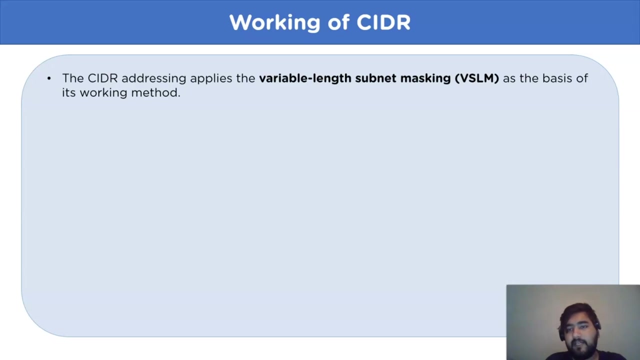 this IP address is 28 and the host ID is 4, which is calculated using 32 minus 28, because in an IP 4 address 32 bit is the maximum limit. Now let's move on to the next heading, that is, working of CIDR. The CIDR addressing applies the variable length subnetting masking, that is BSLM for short. 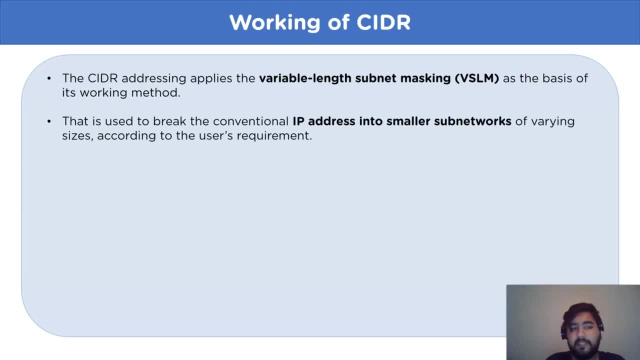 as the basis of its working method. That is the variable length subnetting masking. that is the method used to break the conventional IP addresses into smaller subnetworks of varying sizes according to the user requirement. Let's take a look at an example to understand the working. 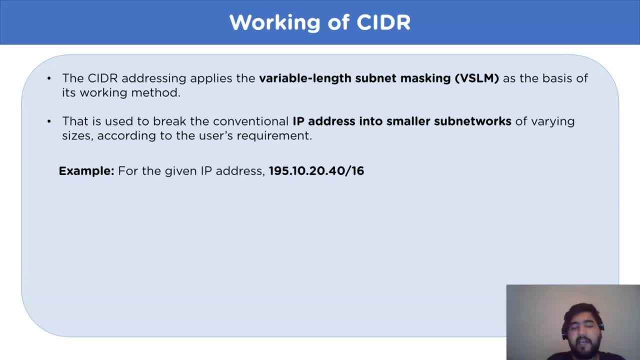 process. In the given example, the IP address is 195.10.20.40 slash 16.. Now let's solve the question. To begin with, from the given IP address we can determine the network prefix, that would be 192.10.20.40, whereas the suffix represent the slash 16 part, The number 16 in an IP address. 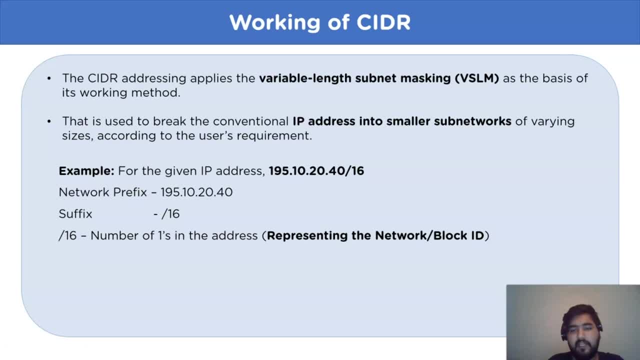 represent the number of ones in the address that is known as the block ID or the network ID, and the host ID is determined using 32 minus 16, because 32 is the maximum limit of bit length in an IPv4 address. So the host ID is 16 and the total number of hosts that are available in the network is 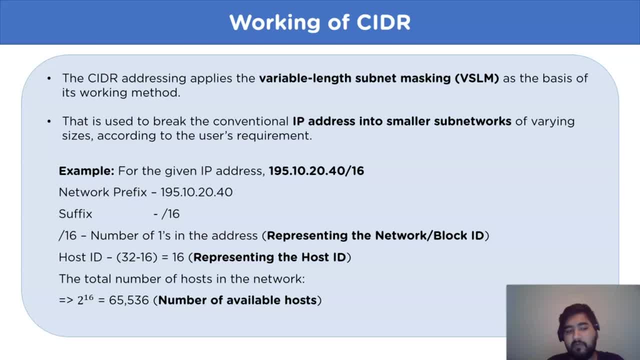 calculated using 2 to the power, number of hosts, that would be 2 to the power, 16 for this case. So the value is 65,536 available hosts in this given network ID. Now let's move on to the examples to better understand the working. 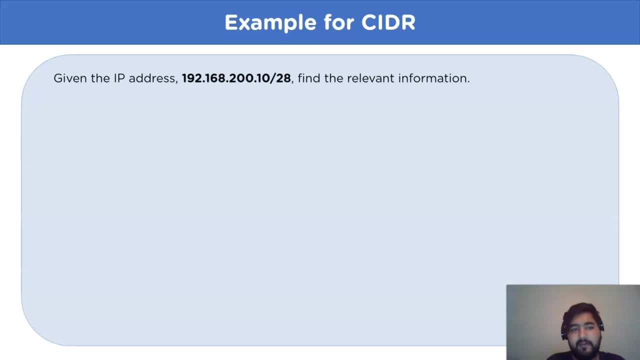 The first example is the given IP address, 192.168.200.10 slash 28, and we have to find the relevant information. Let's begin For the first step. convert the IP address in a binary decimal format. that is, for this IP address it would be the given binary format. Now let's find out the network mask for. 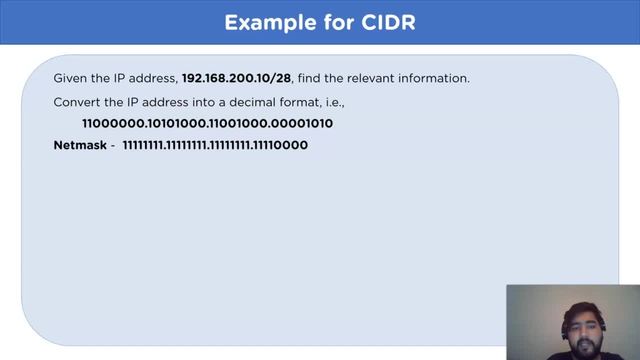 this IP address, that would be 28.1.. the result of the representation is that in this example we have 8 1s and 4 0s. The point to be noted is, according to the slash number, the point, the number of ones for network mask. 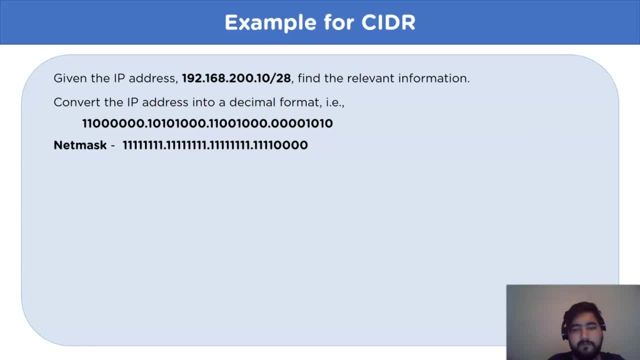 For example, in this question we have slash 28, so the network mask has 28 1s, beginning from left to right, and the last 4 digit would be 0. And in numerical form the value comes out to be 255.255.255.273.4. 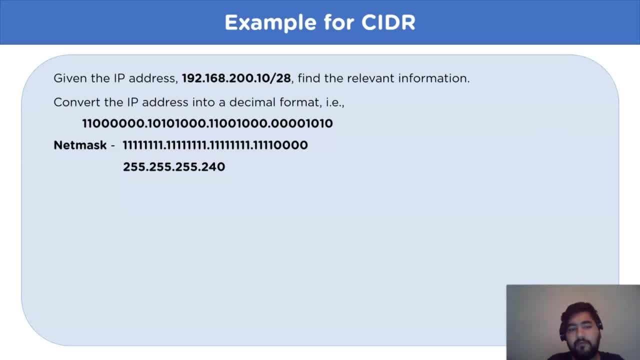 15.355.255.265.0 and 255.255.255.274, 15.355.255.264 and 255.255.274, And this is the network mask for our IP address. Now let's move on to the next information, that is, network ID. 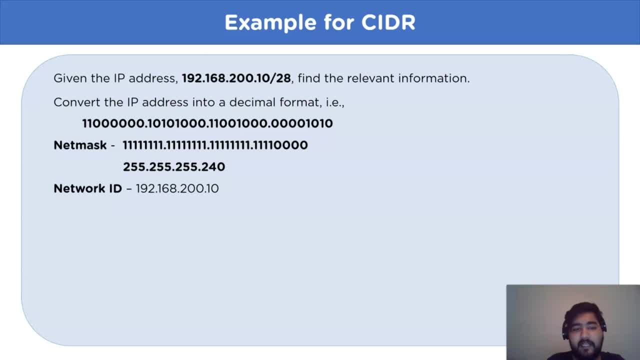 The network ID for the given IP address is calculated using this way, By the given subnet mask, that is, slash 28. we assume that 192.168.200 does not change because it is a part of network ID, And the point to be noted is the network ID is never to be trampled with.